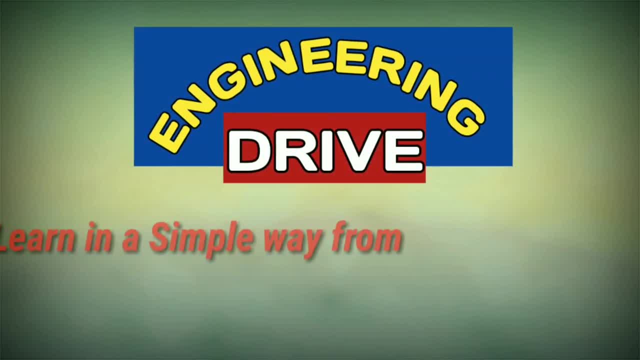 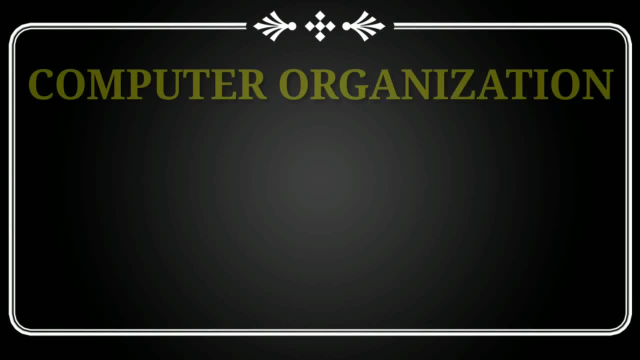 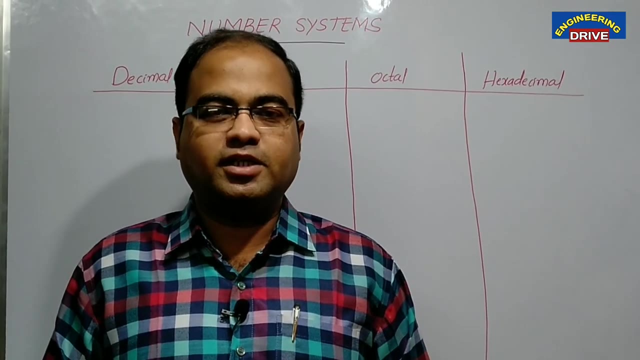 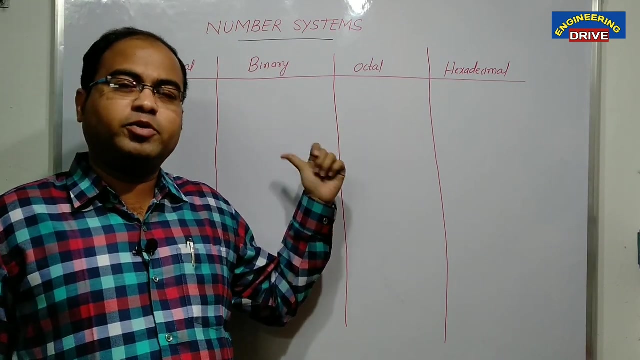 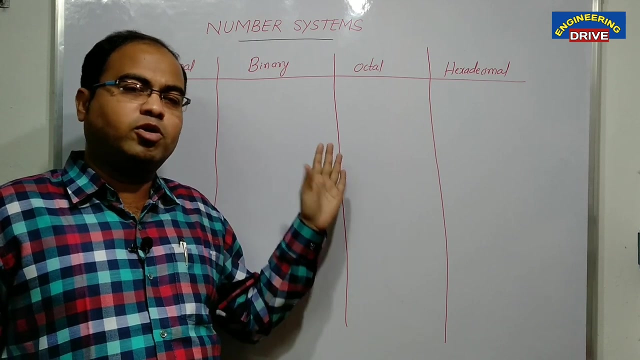 Hi everyone, this is Atik. Welcome to my channel, Engineering Drive. Today I am going to discuss one important topic of subject, computer organization as well as this concept is so popular that this- the questions belonging to this concept- has been appeared in many competitive exams. 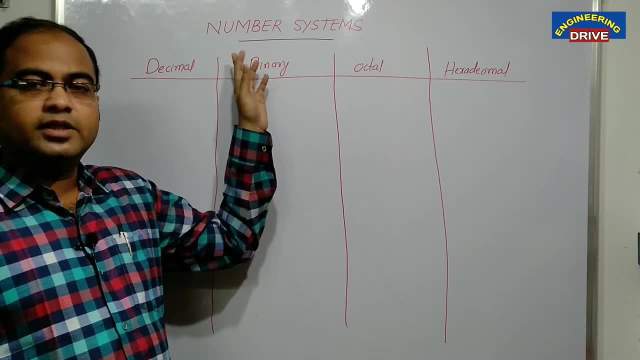 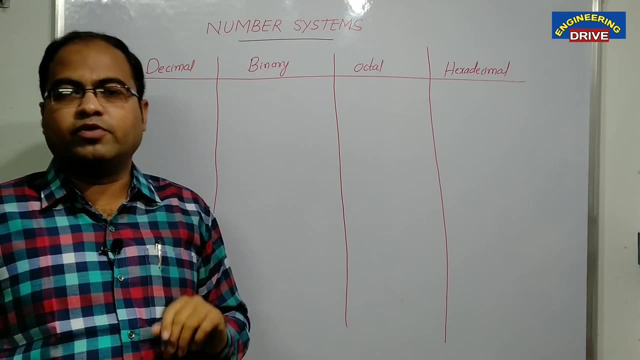 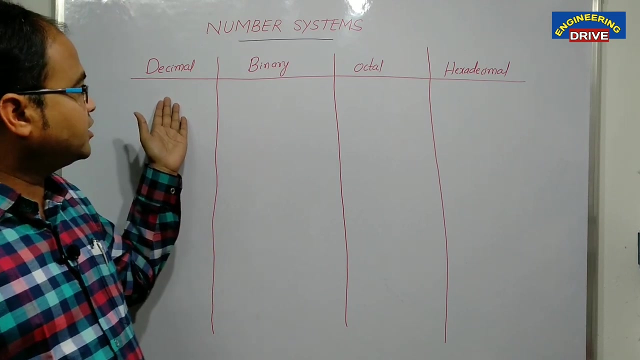 as well. So the topic that I am going to discuss today is number systems, which is very, very popular concept. A computer can represent the numbers in four different ways. Number is same, but it can be represented in four different ways. One is decimal number system. 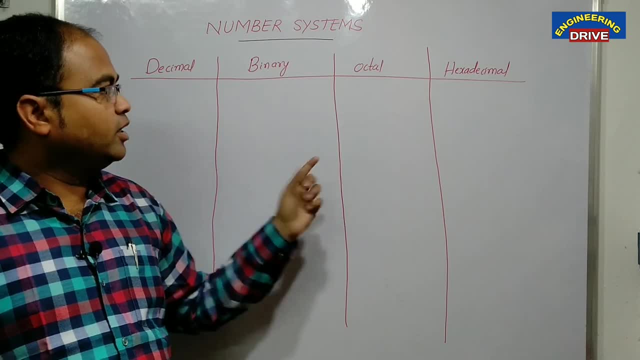 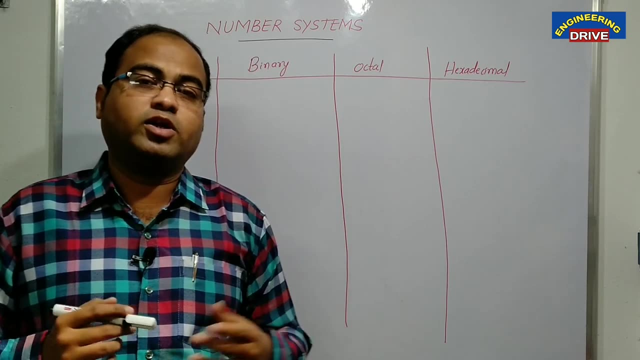 binary, octal and hexadecimal number systems. You will take one number. that number can be represented in four different ways. So how our computer represent those numbers in four different ways. And as a user, if in exams I just now I told you that it is not, 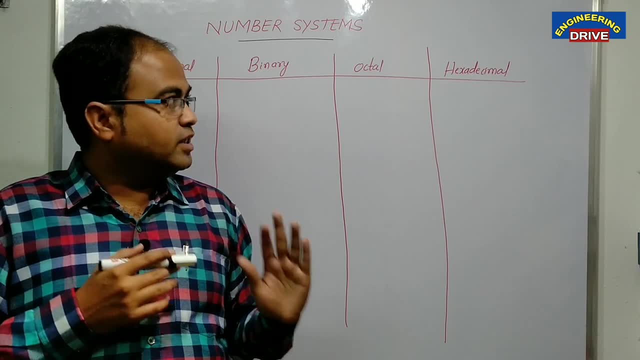 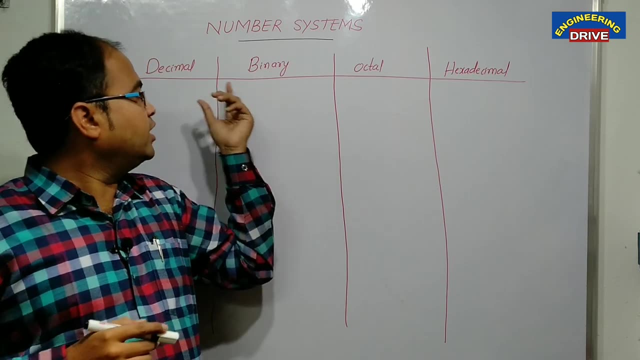 a subject related concept. but also this concept has been asked regularly in many competitive exams. How they will ask the question means they will give, let us say, one decimal number and they will ask you to convert into binary. or sometimes they will give octal number and 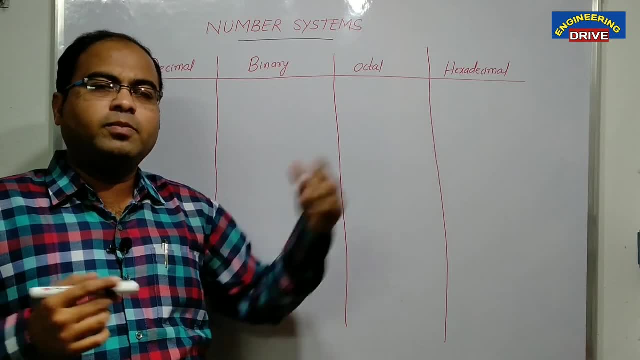 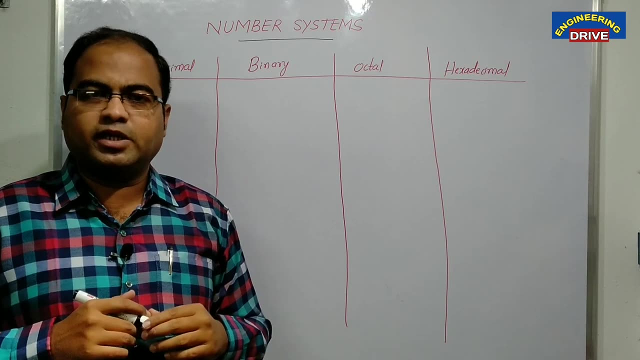 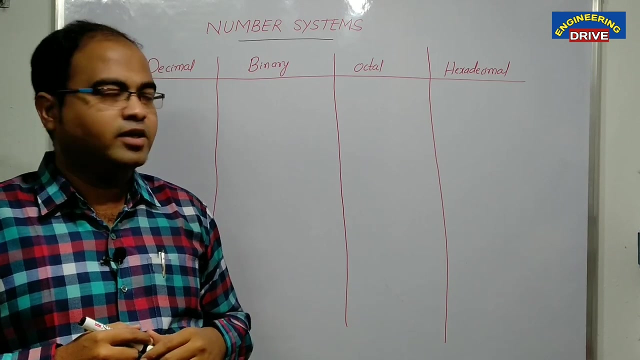 they will ask you convert into hexadecimal number. Okay, so people will face generally a lot of complexity in order to solve this type of problems, But today I will be presenting you one simple method in which you can convert one representation of number into another representation very easily. Okay, as we know, 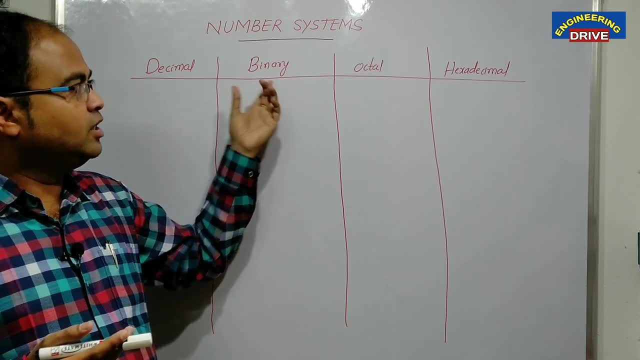 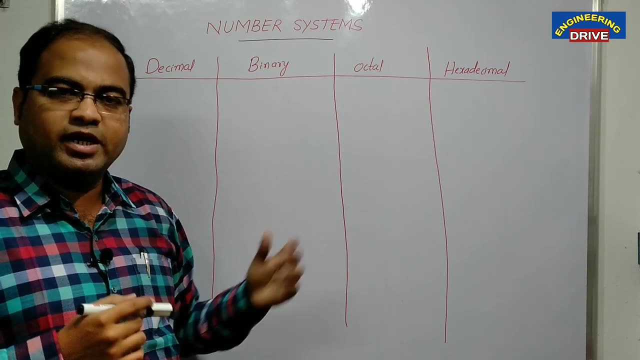 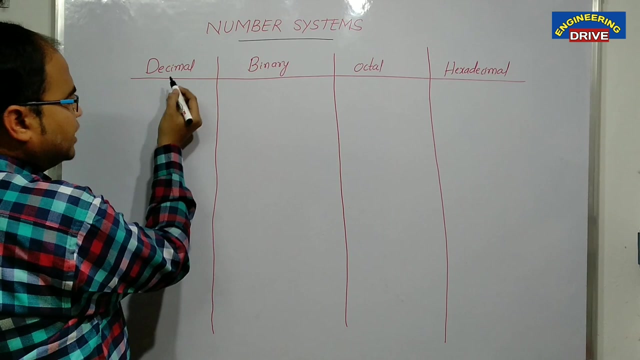 that our computer understands. machine language is a binary language, But along with that binary language we can represent the numbers either in decimal, octal or hexadecimal number system. Okay, let us start the conversion. Let me take one number. decimal number means actually general numbers which we can understand. 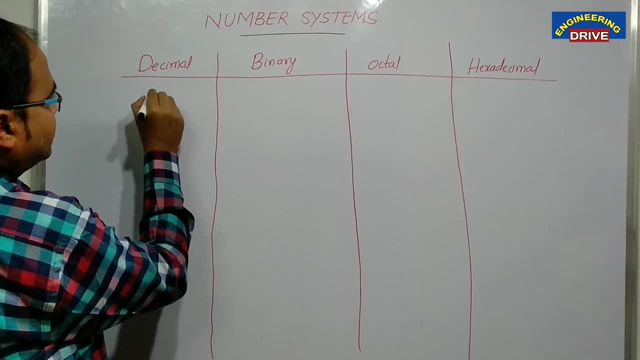 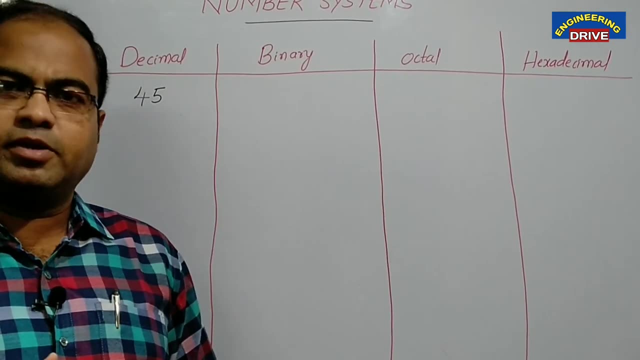 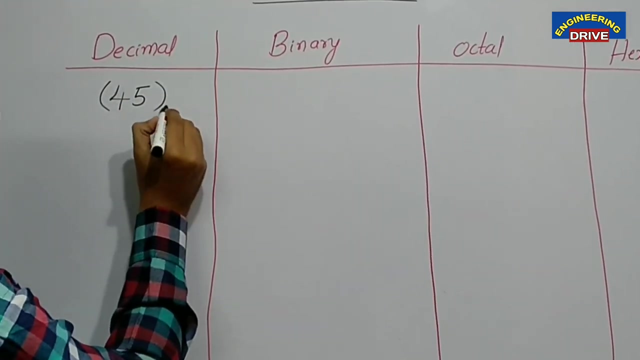 Okay, let us say we will take one decimal number: 45. So 4512300000. they are all decimal numbers. First of all, we should know one thing: a decimal number will have a radix 10. What is the radix? I will tell you. binary number: We don't know what is the binary number. 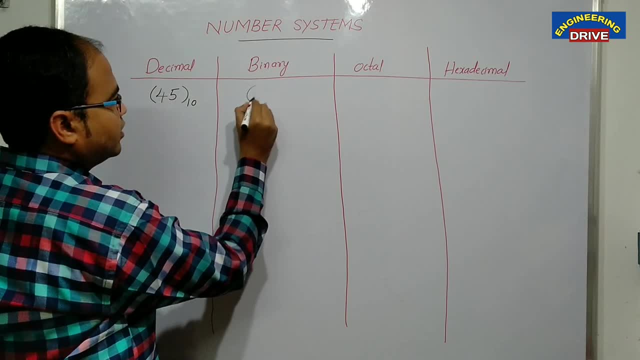 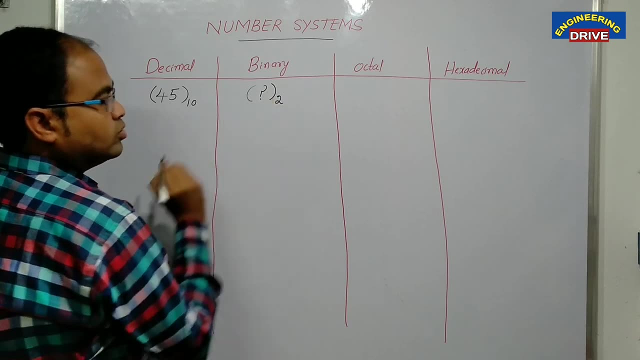 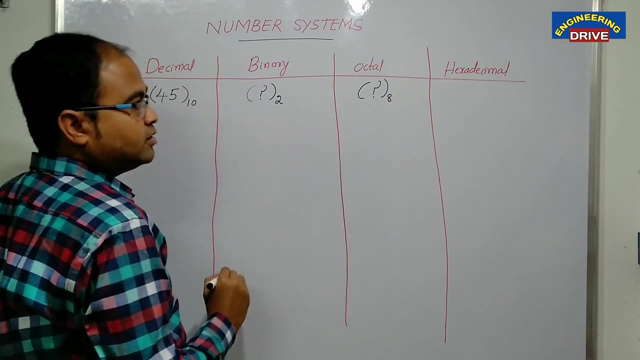 What is the binary number of this 45 representation? Just for our simplicity, I am keeping question mark. binary number will have radix 2.. Octal number: we don't know the actual octal number. Octal number will have the radix 8 and the last one hexadecimal number, will have the 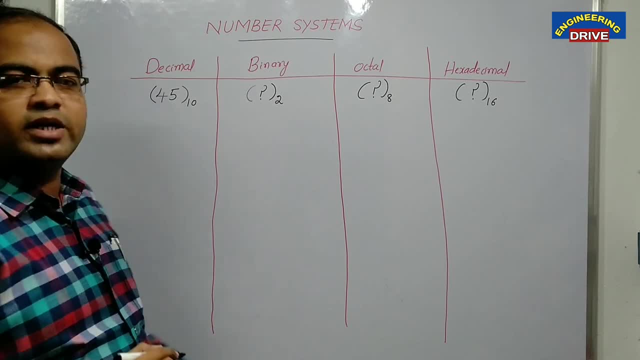 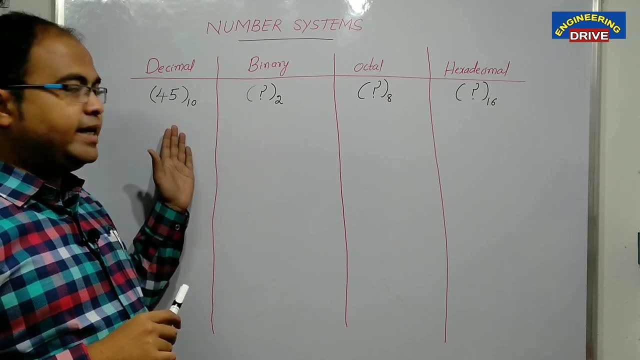 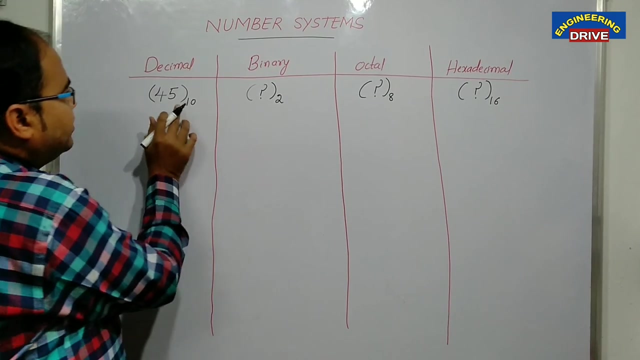 radix 16.. Sir, what is the meaning of radix now? Radix is very, very important part of every representation. If we know radix properly, then easily we can convert one number to another form, another number representation. Okay, now what is the meaning of radix 10? 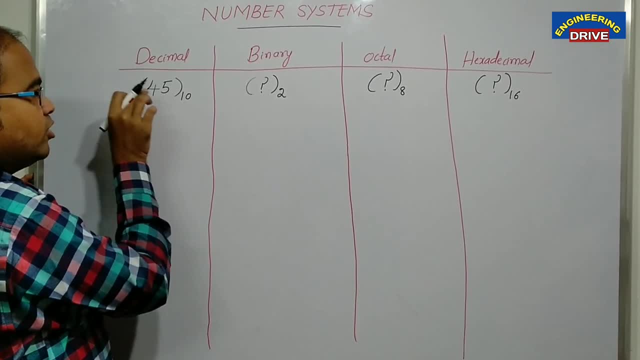 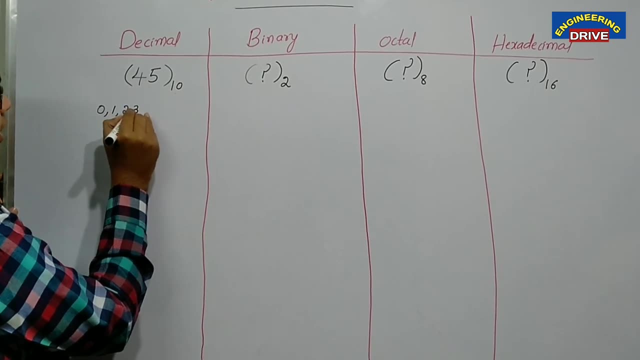 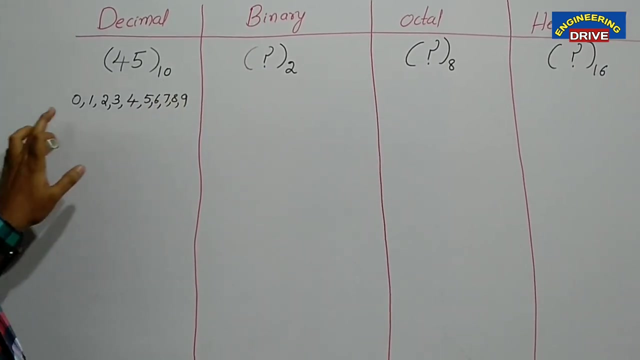 here for decimal number. Radix 10 indicates, in order to represent decimal number, we can use the digits 0 comma, 1,, 2,, 3,, 4,, 5,, 6,, 7,, 8 and 9.. So if you count zero to nine, you 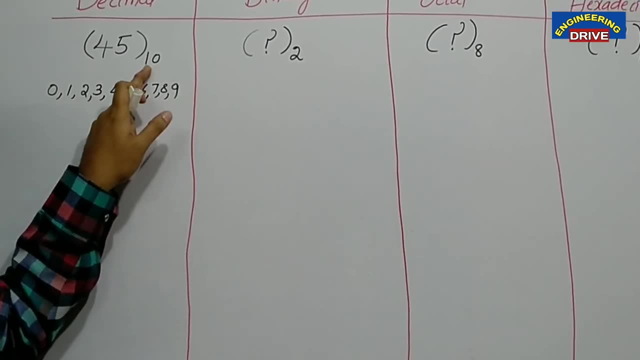 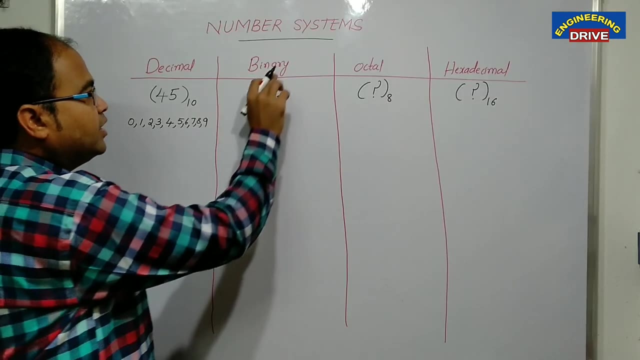 can use the digits from zero to nine. How many numbers are there? Totally, 10 numbers are there, So radix is 10.. To represent this decimal number, you can use the digits from zero to nine. Okay, Similarly, to represent binary numbers, how many digits you need to? 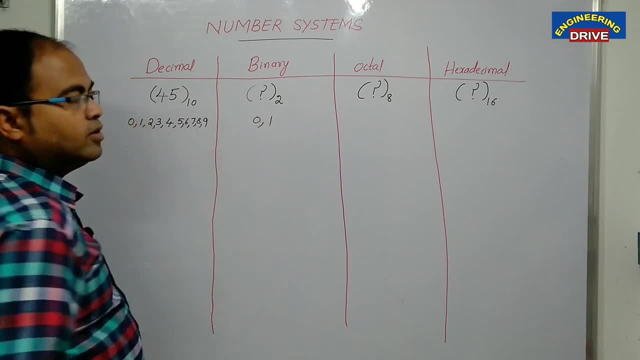 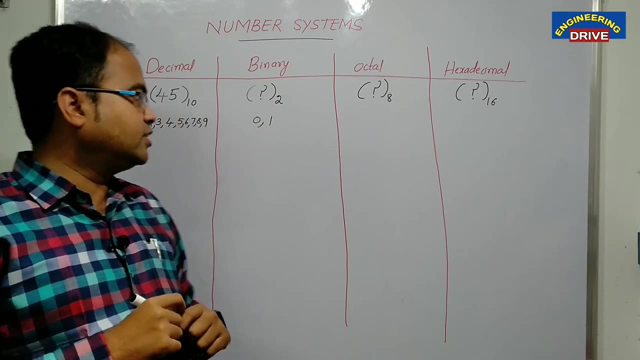 use Only two digits. Those are zero and one. That's why the radix of binary number is two, because to represent binary number, we will make use of only two digits. Similarly, for octal, to represent octal number, how many digits you need to use? 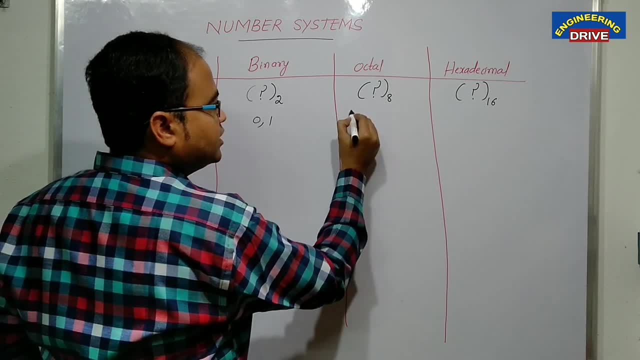 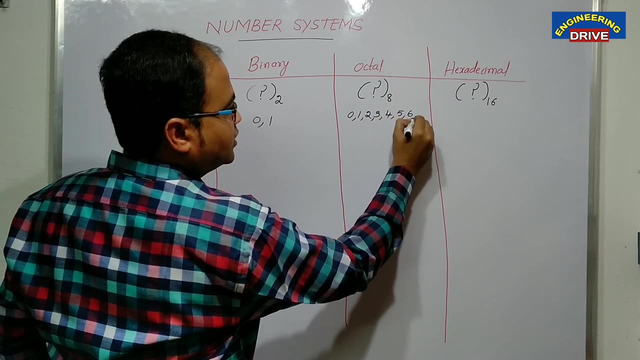 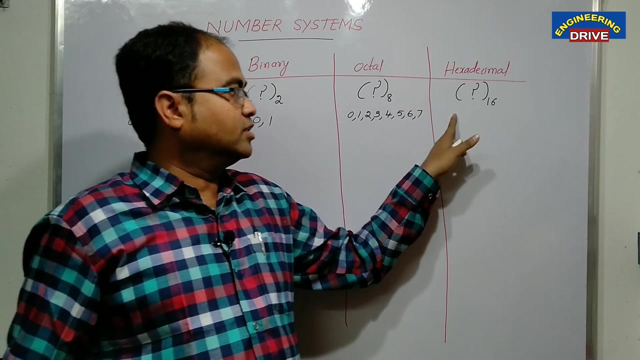 We can use maximum How many digits? Eight digits. So what are those digits? Zero comma, one, two, three, four, five, six and seven. So zero to seven, eight digits. And to represent hexadecimal number system, you know hexadecimal number, radix is 16, which means how many digits. 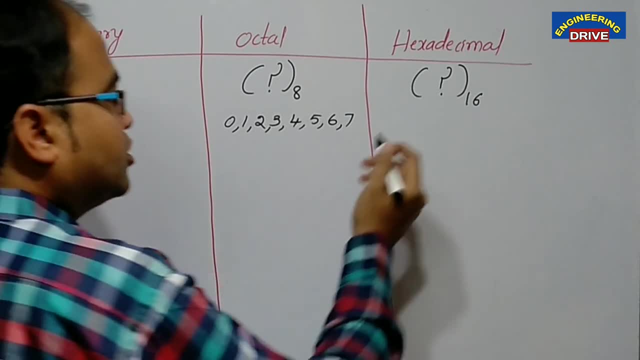 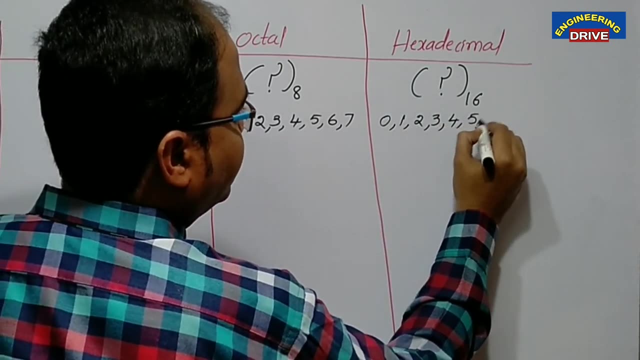 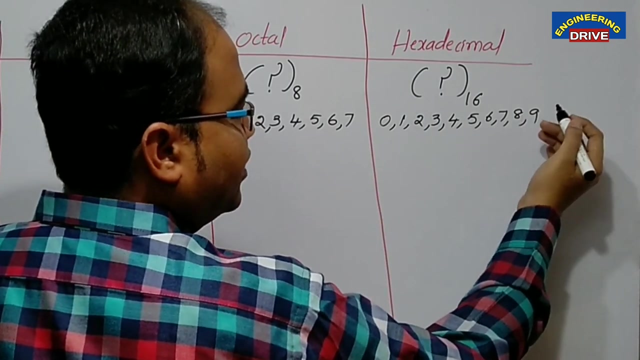 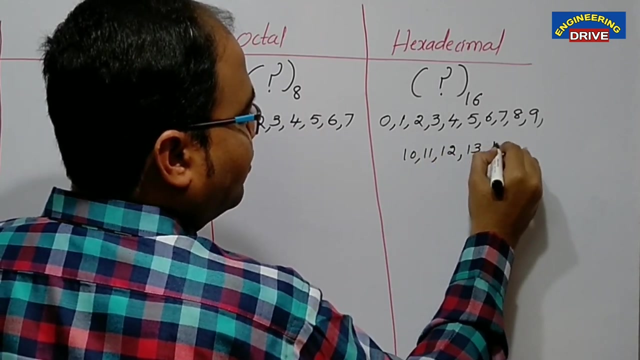 we will use 16 digits. we will use. So what are those digits? Zero comma one, two, three, four, five, six, seven, eight, nine from nine- slight change: What? generally, after nine, what will come? Generally, we will get 10,, 11,, 12,, 13,, 14 and 15.. These are the 16 digits. 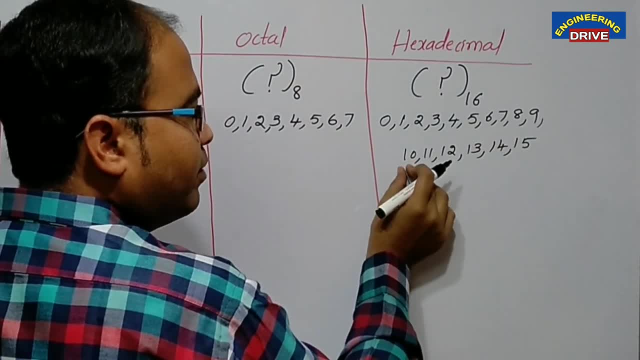 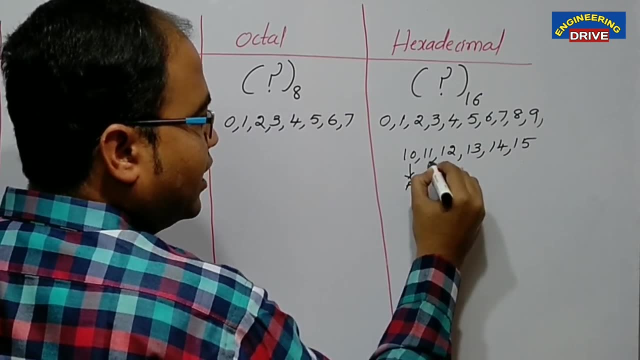 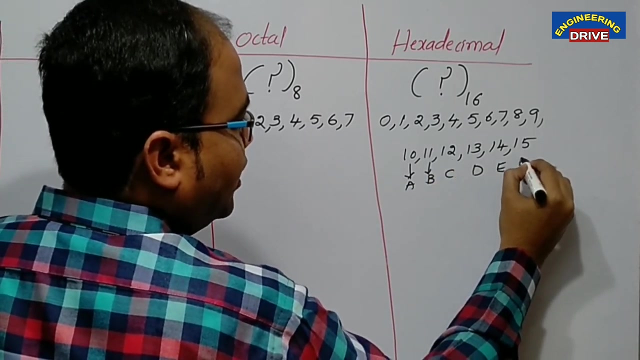 But for hexadecimal number system, slight change from up to nine. It is okay as it is. you write down from 10.. 10 is represented A, 11 is represented with B, 12 C, 13 D, 14, E and 15 F, which means a hexadecimal number. 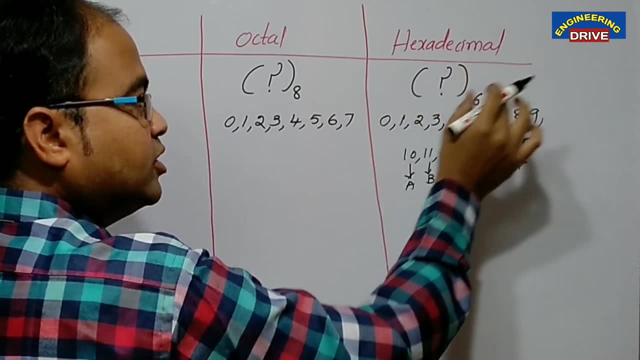 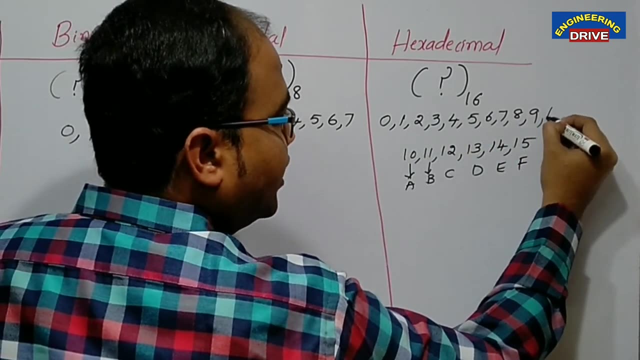 system. The radix 16 means you can use 60 zero to 15 numbers, That is totally 16 up to nine, It is same. But after nine what you should do? Write down A comma, B comma C, D, E and F. 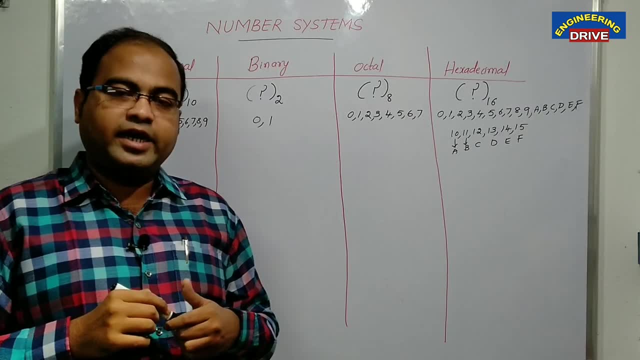 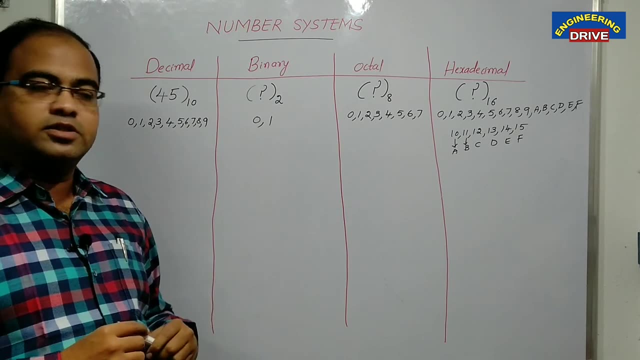 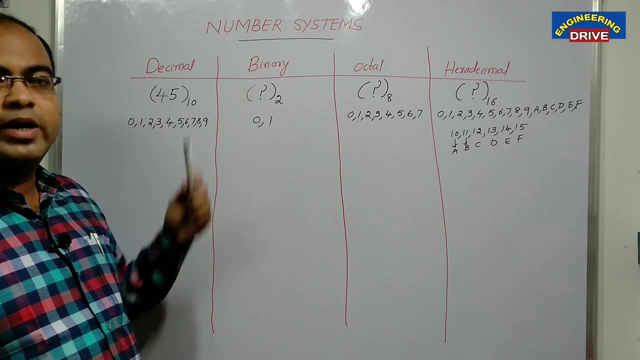 That's all. So these are. this is the. it is the clear explanation of radix. Now, if you know radix properly, then easily you can solve all this conversions. Let us say I have taken a decimal number, 45. How I can convert this decimal number into binary number? Okay. 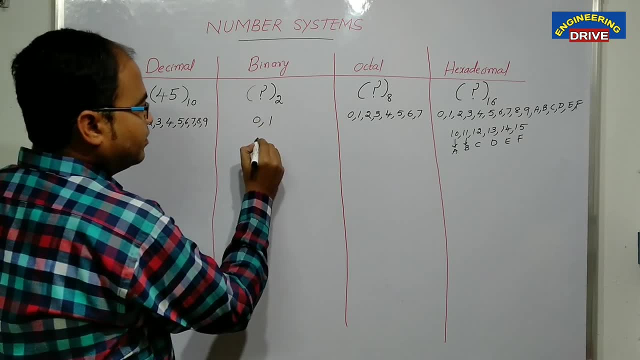 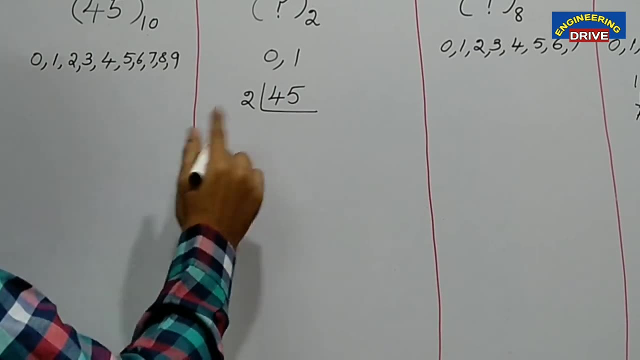 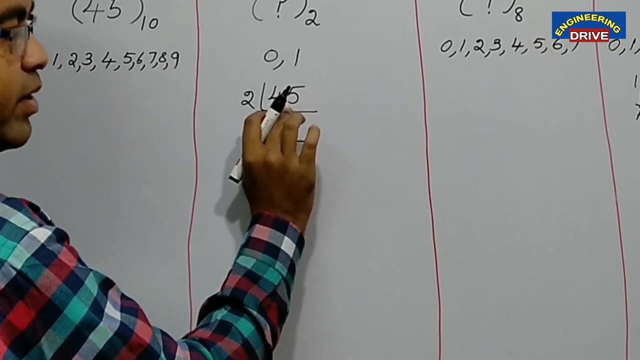 What is the radix of binary number two? So take this decimal number 45 and divide it with two, That's all So, which means 222, you will get 44. That actual number is here 45. So how many number? 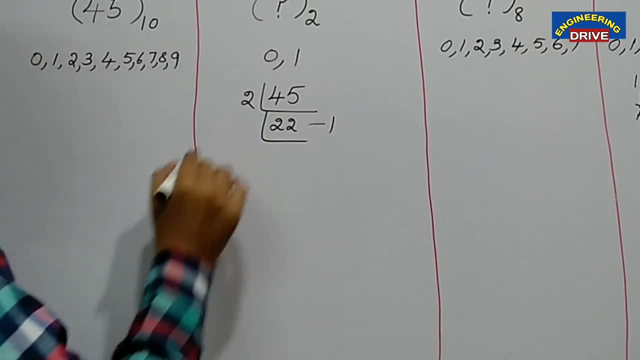 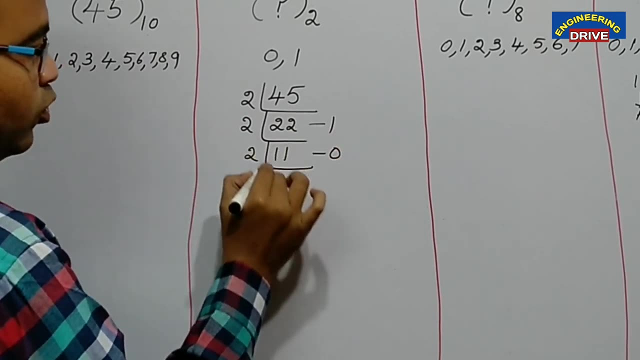 will remain. if you subtract, One number will remain Okay: Next 2, 11, 22.. Any number will remain No. That's why you write zero: Next 2, 5, 10.. So any number will remain Yes. 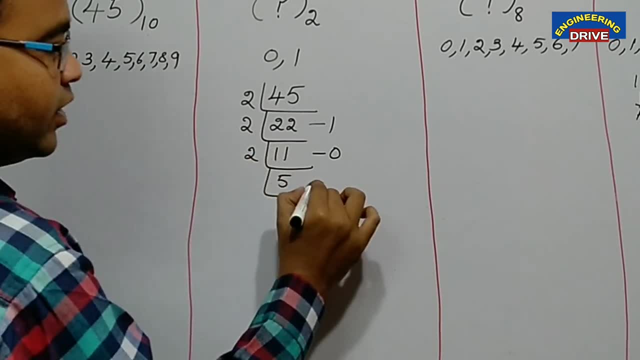 one number will remain: 2, 5, 10.. But actually it is 11.. 11 minus 10, 1. 1.. Next, 2, 2, 22.. Any number will remain No 4.. Any number will remain. One number will remain Next. 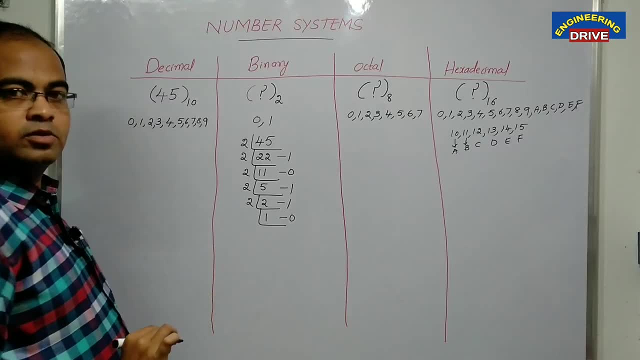 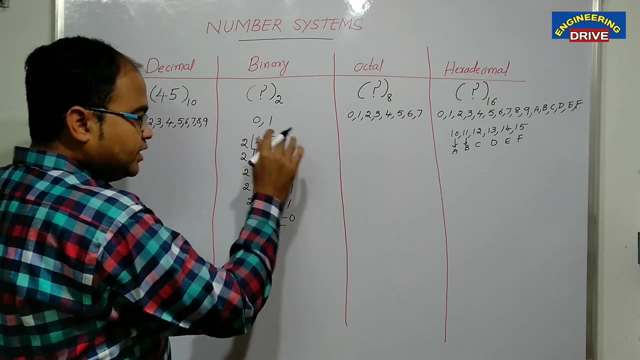 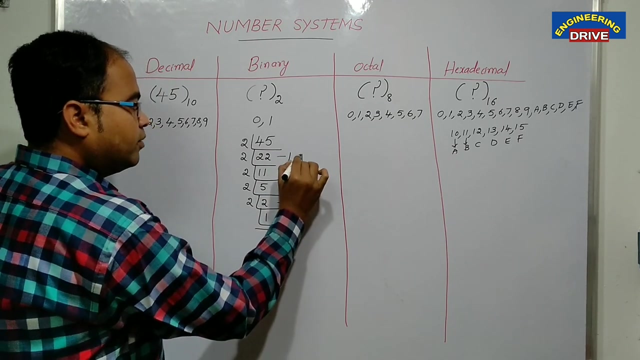 2, 1, 2.. Any number will remain No. So you stop your problem. now here You stop your simplification. Now how to? this is everything we got in: ones and zeros. So how we should write the answer: Write down from bottom to top, Don't write from top to bottom bottom. 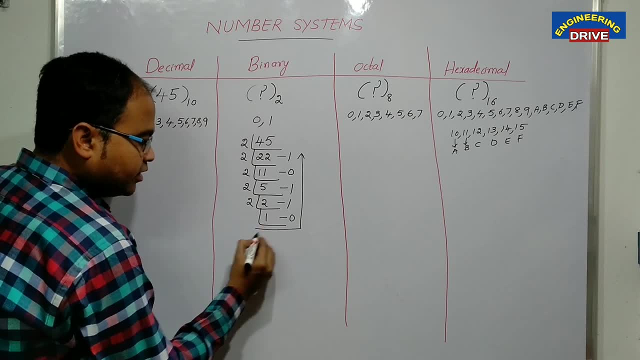 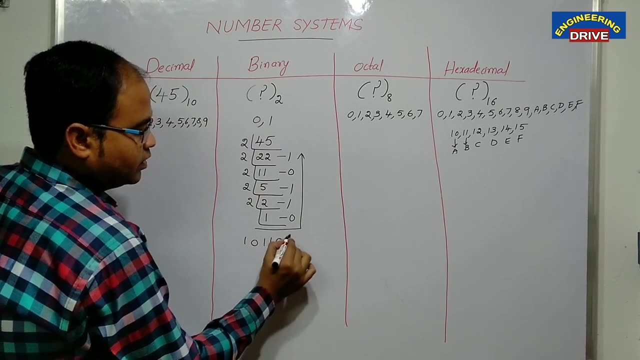 to top So bottom. to top what you will get Write down here: One zero four. One zero one. One zero one. One, one zero one. So this is our binary number. Okay, This is. 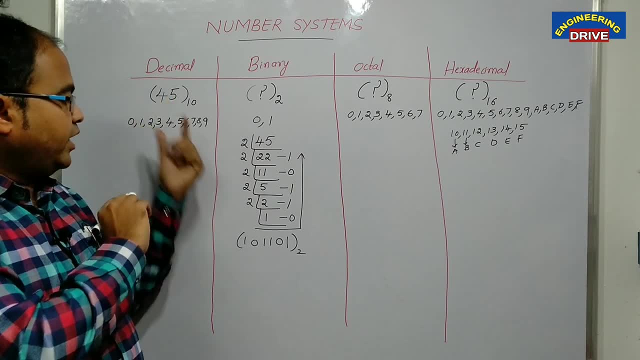 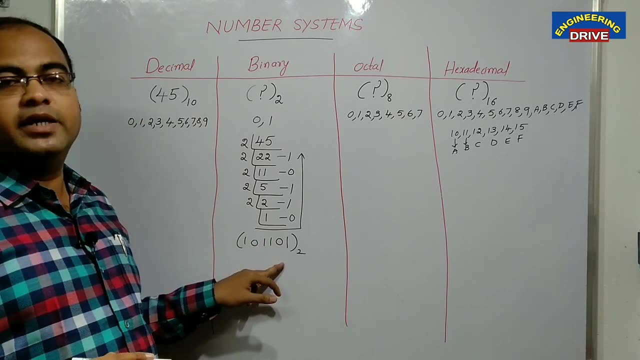 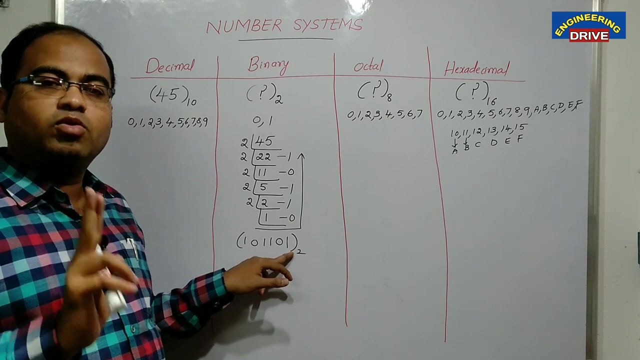 equivalent to that of 45.. 45 and one zero one, one zero one. both are same. The only difference is this is a decimal number and this is a binary number. Now you can see why we have written radix 2, because this binary representation makes use of how many digits. 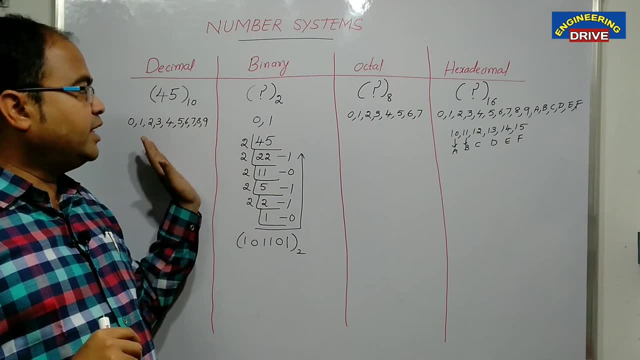 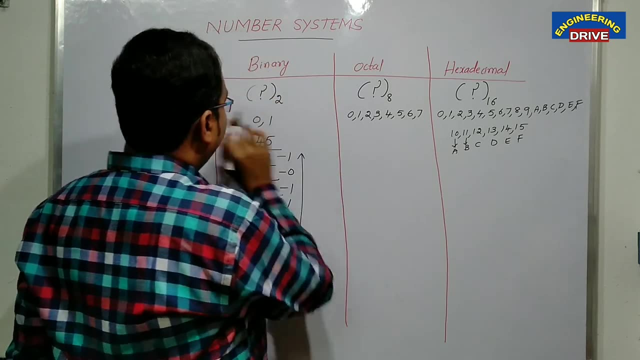 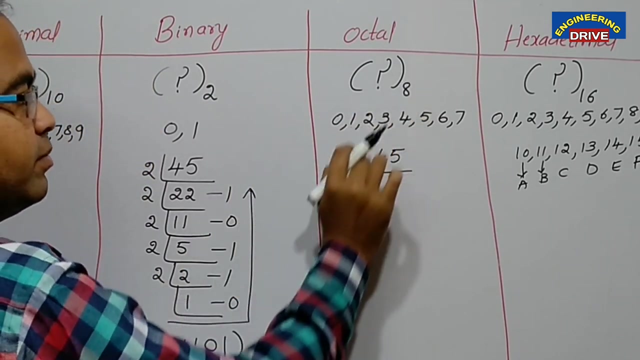 Only 2 digits. We have converted decimal number to binary. Now let us convert decimal number to octal now. So how to convert decimal number to octal? Take the decimal number 45 and you need to divide this decimal number with- yes, very good- with radix 8.. So 8.. Okay, What we will? 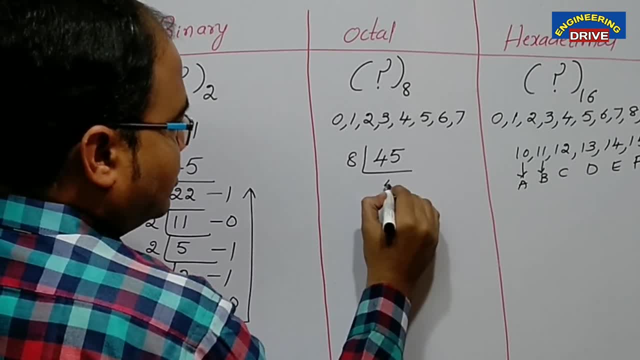 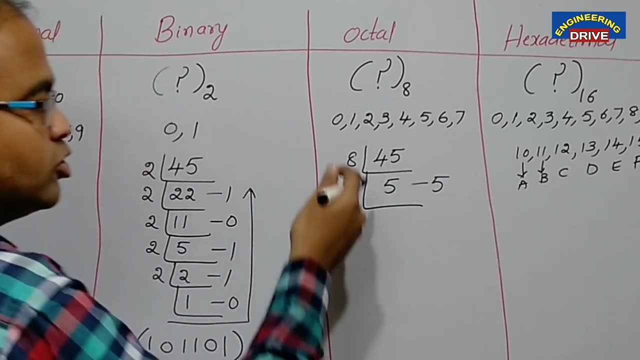 get 8, 5, 40.. 8, 5, 40. So 45 minus 40, how much 5.. So we can't simplify it more now because already we got the last. we came to the end. 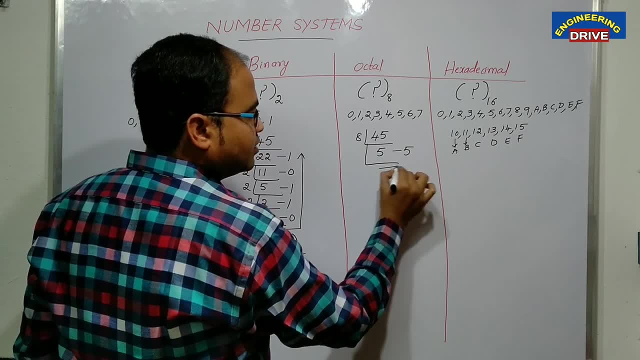 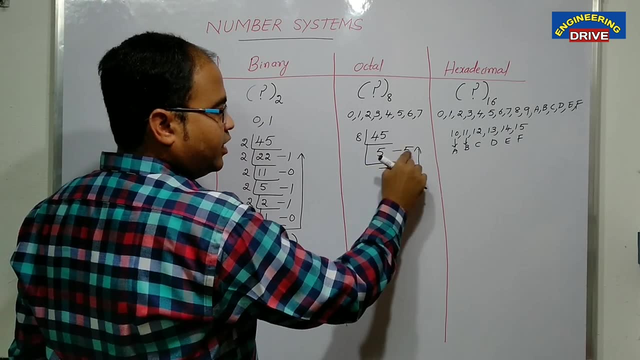 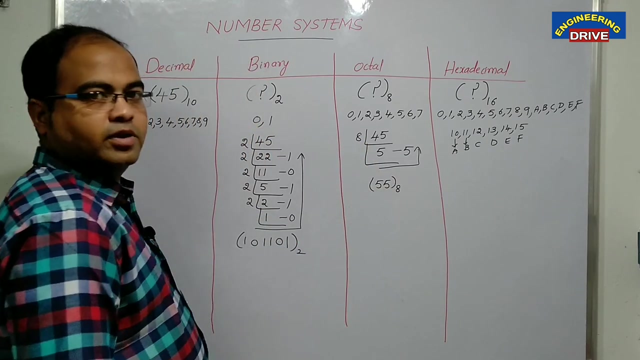 of the simplification So directly. how to write the answer Top to bottom. So sorry, bottom to top. Bottom to top means write down like this: 5, 5.. So we got answer double 5.. And what is this octal number? How to verify whether our answer is correct or not? You? 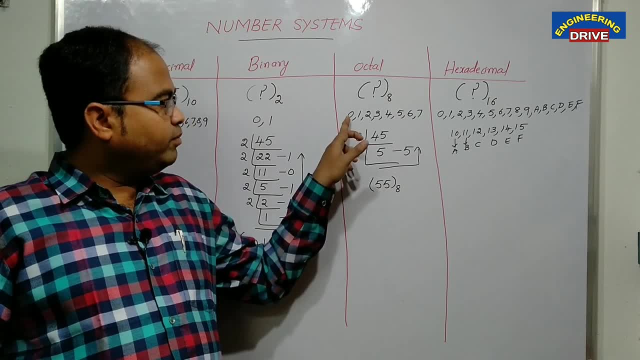 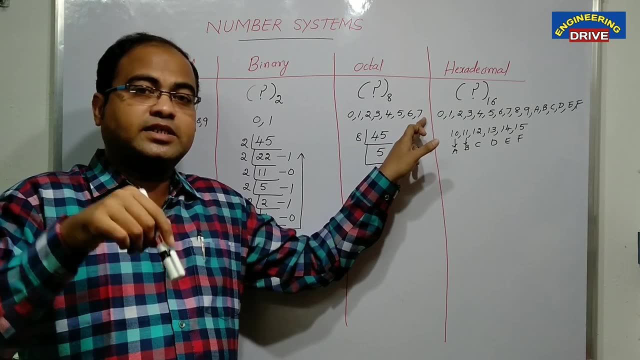 can see that We got 2 digits. Both are 5 and they belong. they belong, of course, to in this range only: 0 to 7 range, only In octal number. if you get any answer such as more than 7, then it. 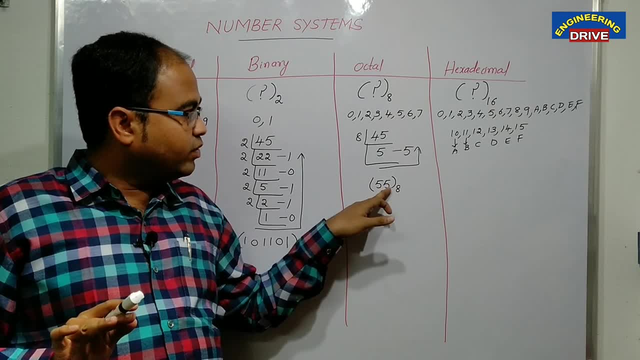 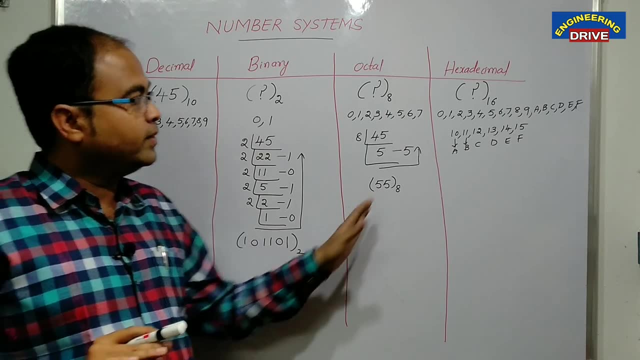 is wrong answer. Remember you should not get that answer. Whatever the answer you will get, it should be within this range: 0 to 7.. Here also binary number 2 digits, zeros and ones only. we got answer. Okay, Now let us convert decimal number into hexadecimal number. 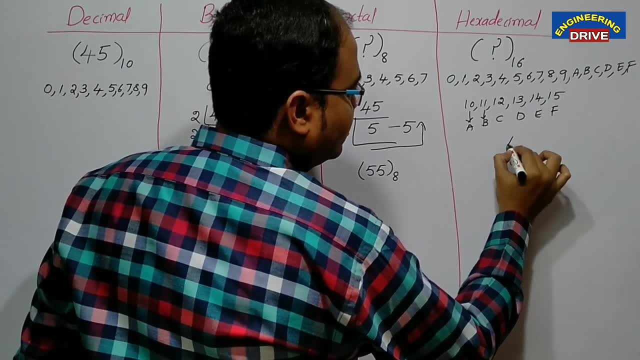 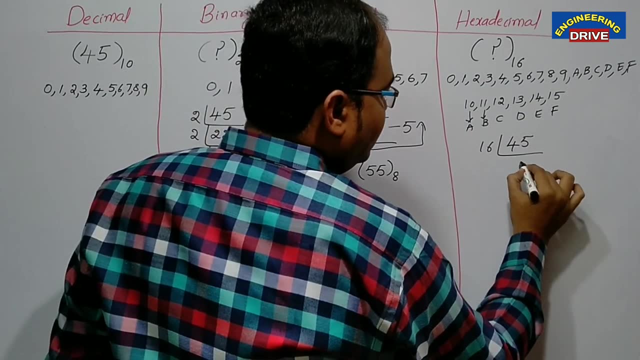 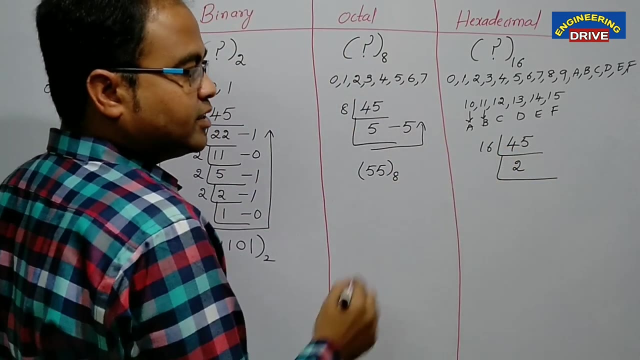 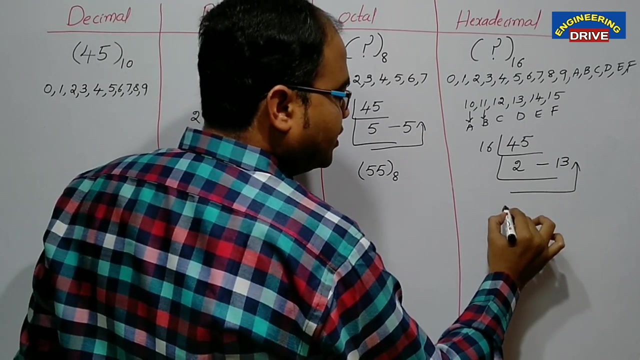 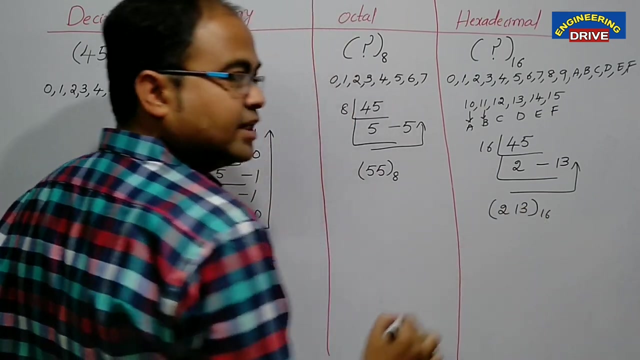 How to convert decimal number to hexadecimal number. We are taking 45 and divide it by 16.. So what you will get? 16, 2.. How much 32? 32.. 45 minus 32, you will get 13.. Okay, So write down answer like this: 2, 1, 3. Whether it is hexadecimal. 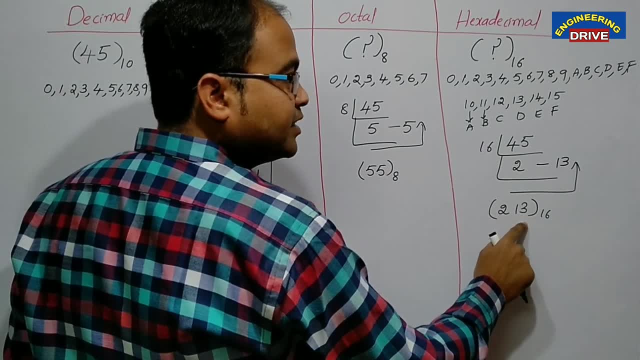 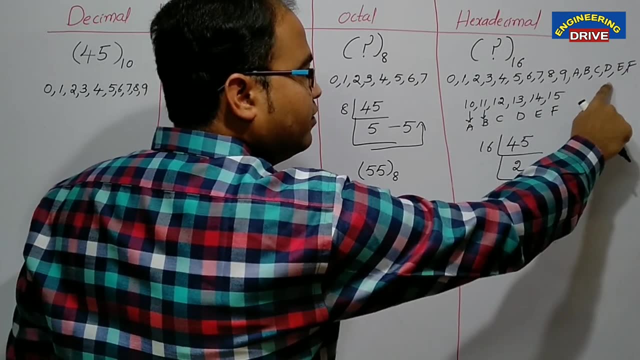 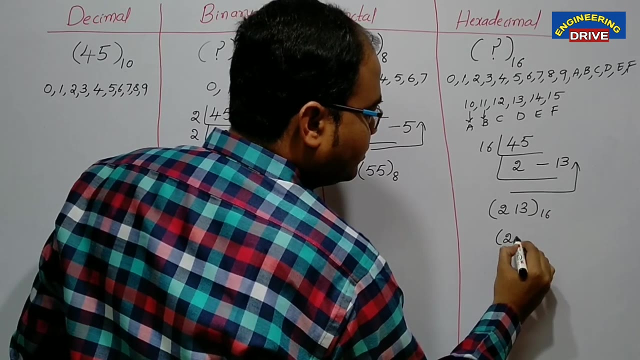 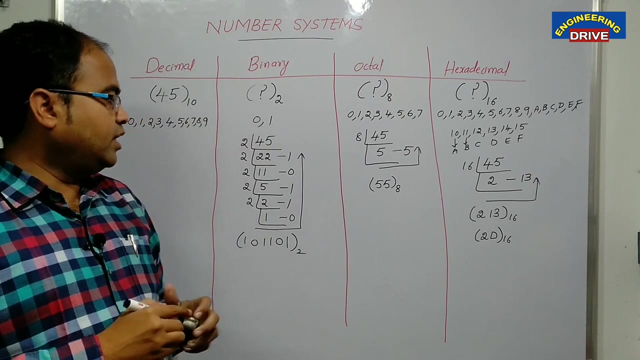 number? No, because 13 we should not represent as it is. from 10 to 15. there is separate representation given for us that only we should take. so what is the representation of 13? 13 representation is d, so write down 2, d and 16. that's all okay. see, here we got the all the three different representations. 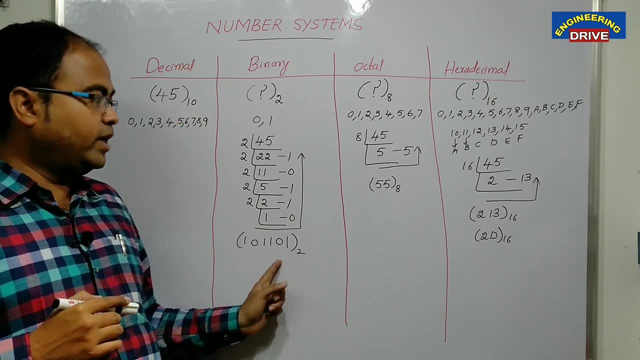 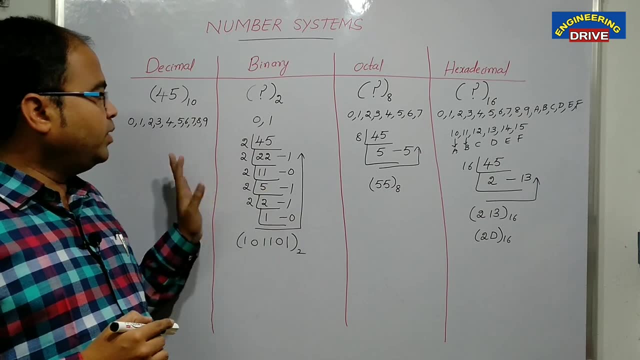 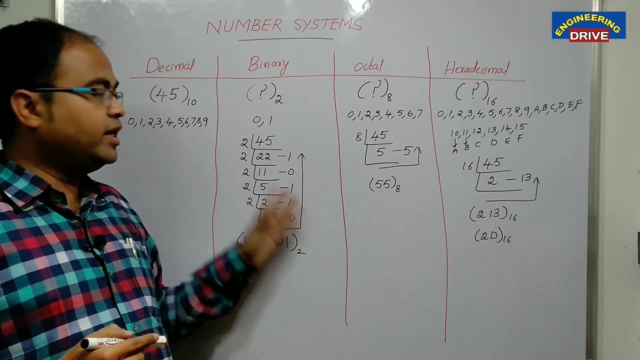 we have taken one number, 45, converted to binary, then converted to octal and then converted to hexadecimal number system. okay, now you people can ask me one question. sir, it is okay, can we convert hexadecimal to decimal, octal to decimal, binary to decimal? yes, it is also possible. how to convert? 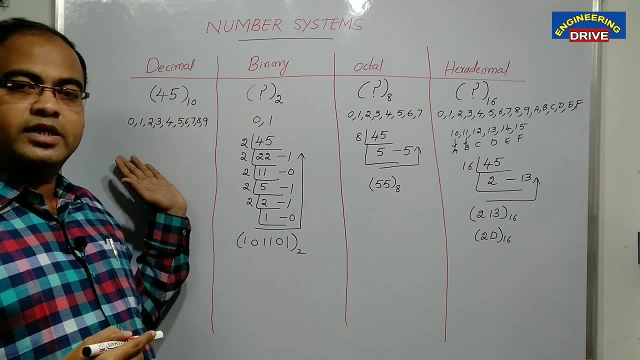 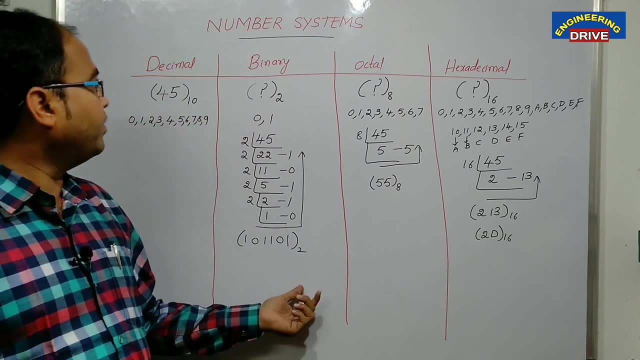 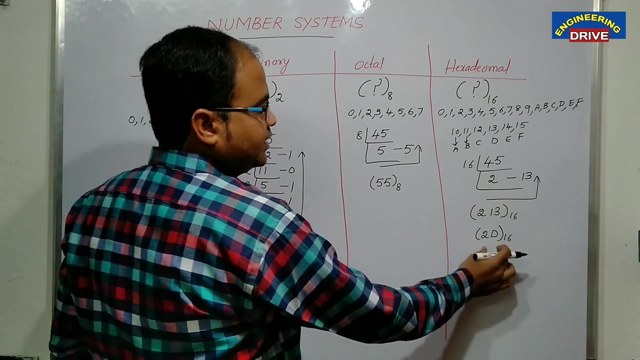 back the these three number systems into back to decimal number system. okay, now let us convert back this hexadecimal, octal and binary into decimal number system. back now, how it is possible? it is quite simple. what we should do means: let us take this is a hexadecimal number i want to convert back into 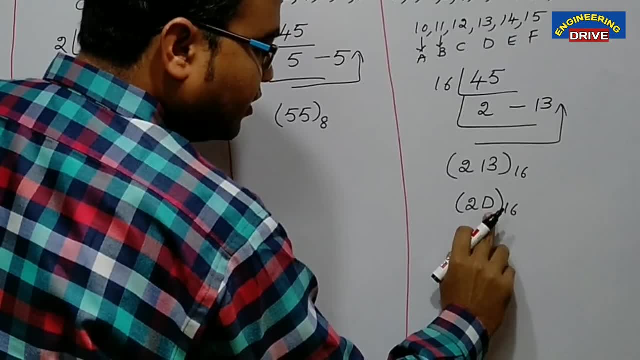 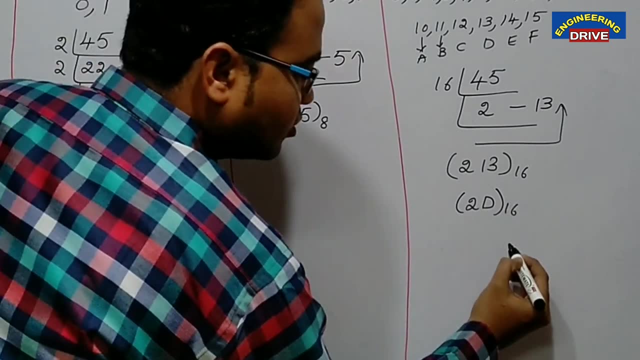 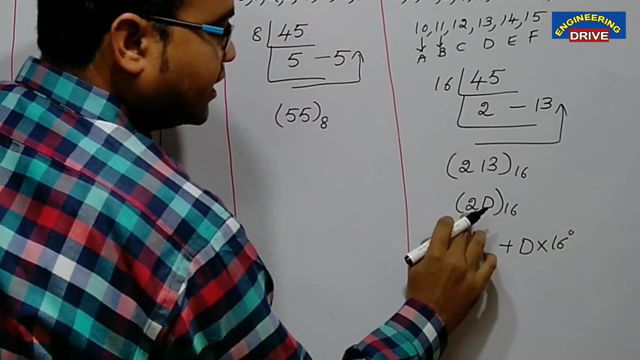 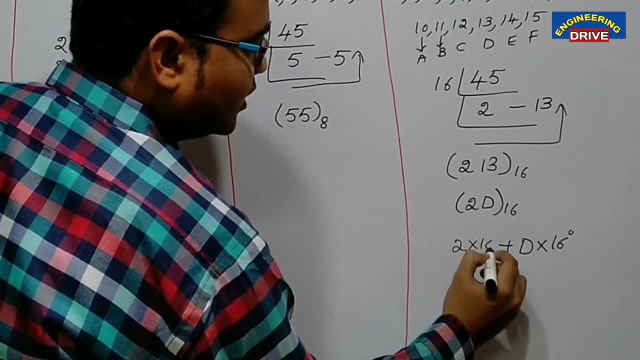 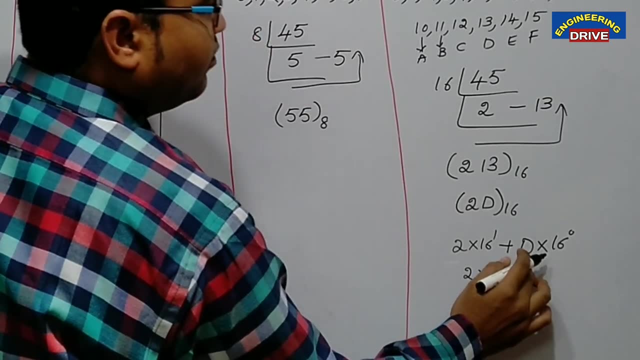 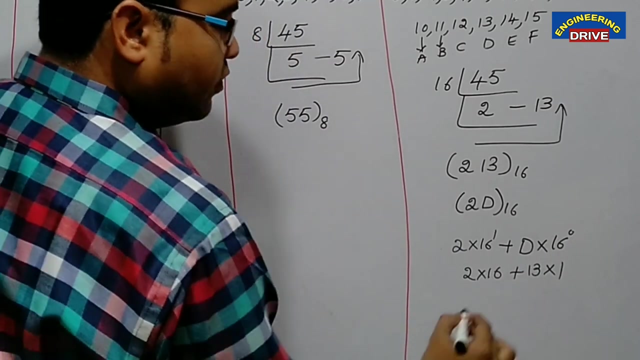 next number: 2 into 16, power 1, so 2 into 16. power 1 means 2 into 16 plus what is the value of d according to hexadecimal? 13, so 13 into 1, so which means what you will get: 32 plus 13, which means: 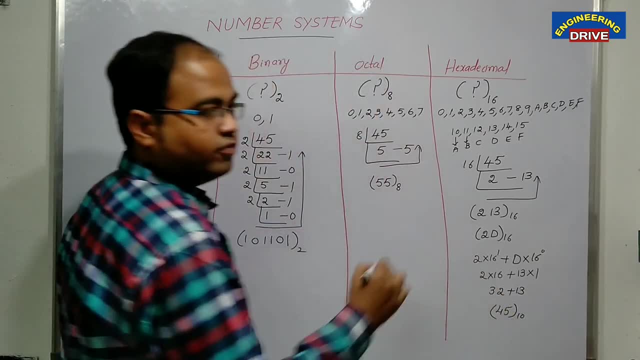 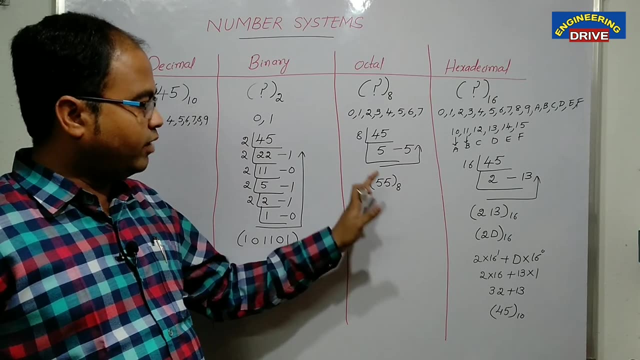 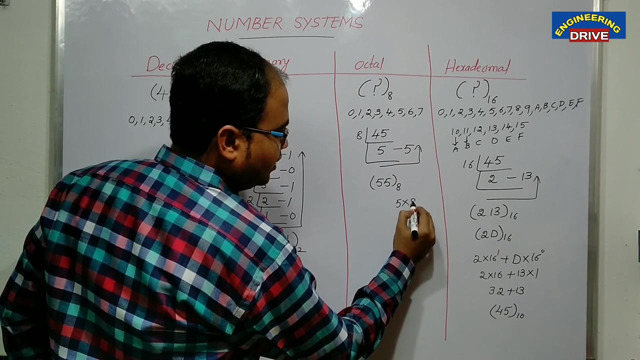 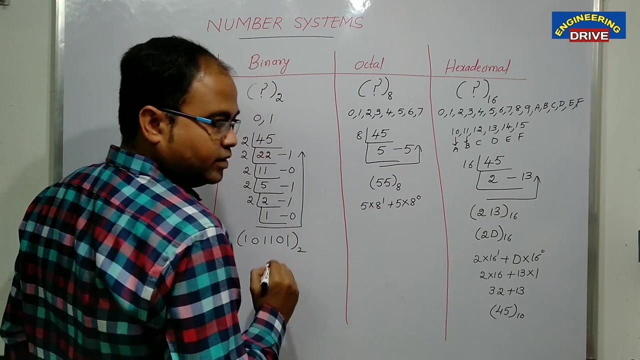 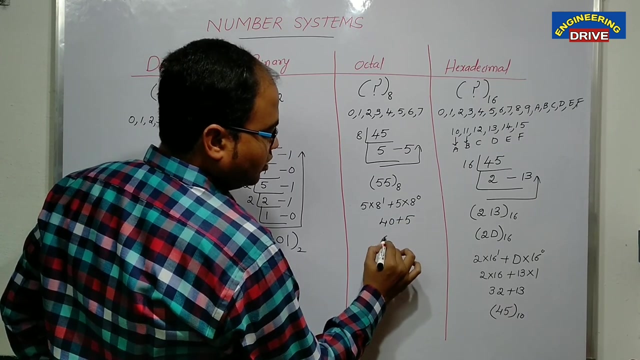 45. 45 is a our original decimal number. okay, same method you use for octal number. also, i want to convert this octal into decimal number. so what to do now? 5 into 8 power 0 plus 5 into 8 power 1. so what i will get? 5 into 8, 40 plus 5. so 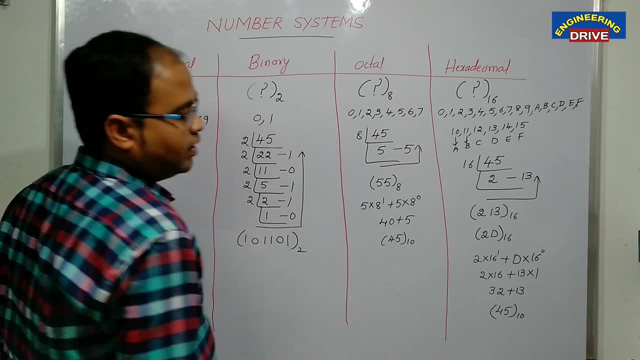 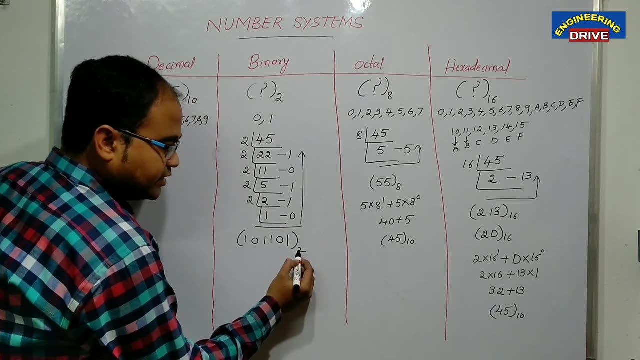 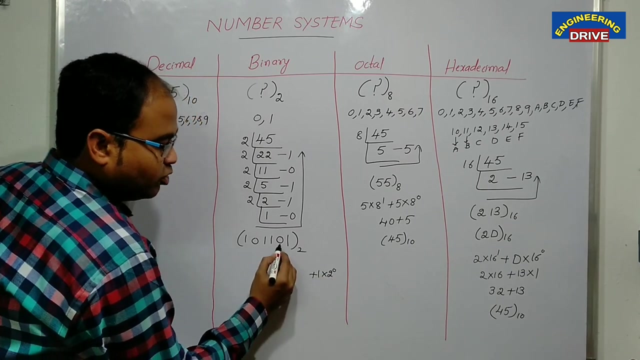 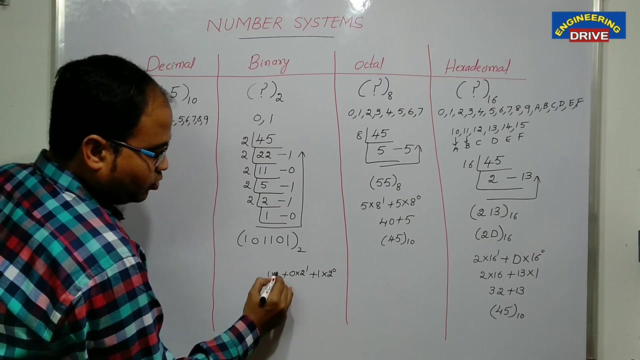 again. i got answer same: 45, which is a decimal number. convert this binary into decimal now, same method. so here, what is the radix 2? you should take now 1 into 2 power 0 plus 0 into 2. power 1, 0 into 2. power 1 plus 1 into 2 square plus fourth one. 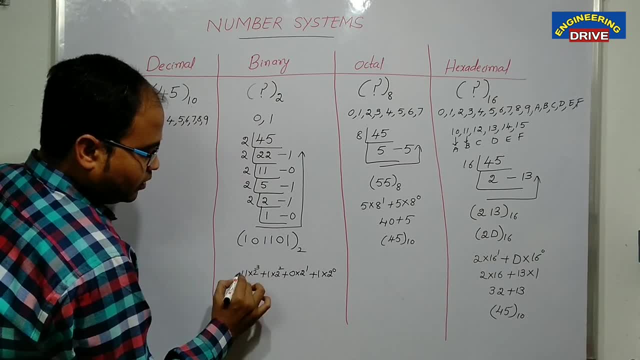 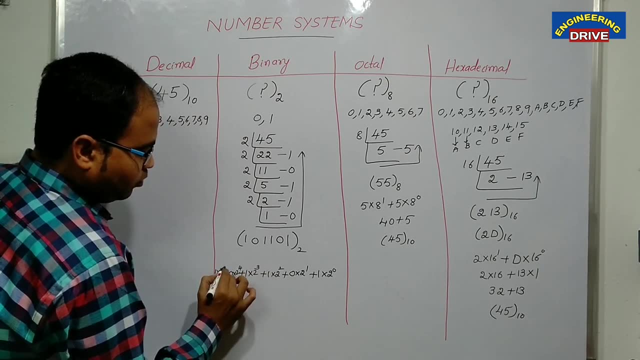 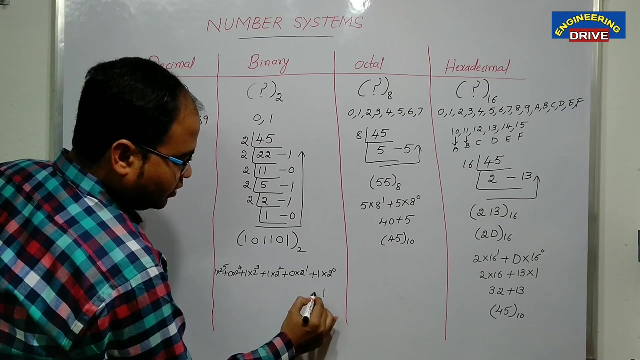 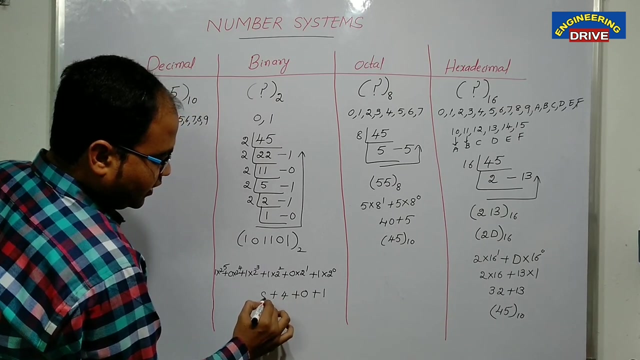 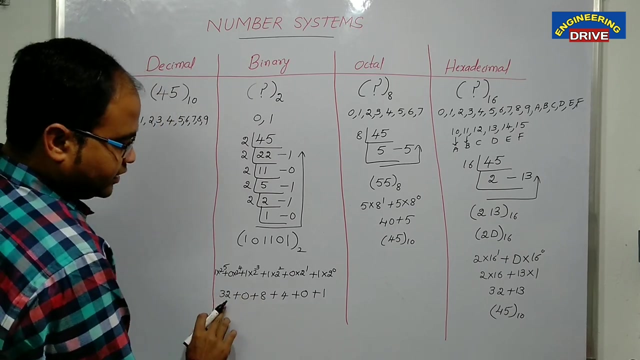 1 into 2 cube plus 0 into 2 power, 4 plus 1 into 2 power 5. so what you will get right down as it is so: 1 into 2 power 0, 1 plus 0 plus 4 plus 8 plus 0 plus this is 32, so what you will get: 32 plus 8, 40, 44 and 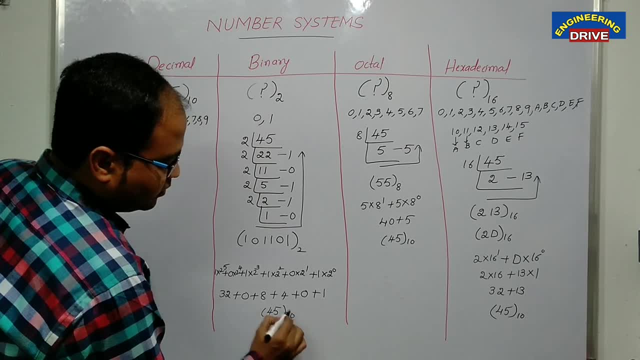 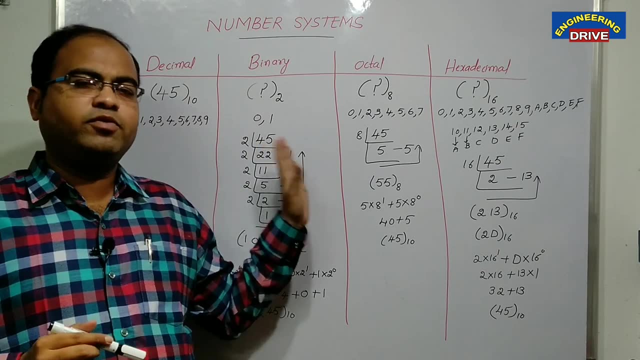 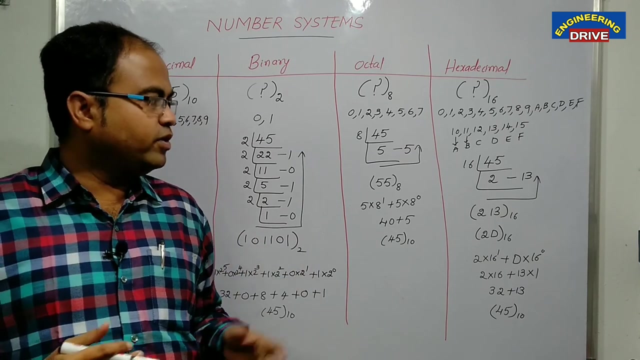 45. again, we got 45, which is also a decimal number. so, my dear friends and students, you know this is quite, a very, very simple method. no matter how many videos you will watch, i don't. i don't think so that there are more number of videos which contain this type of simple methods. this is quite a simple. 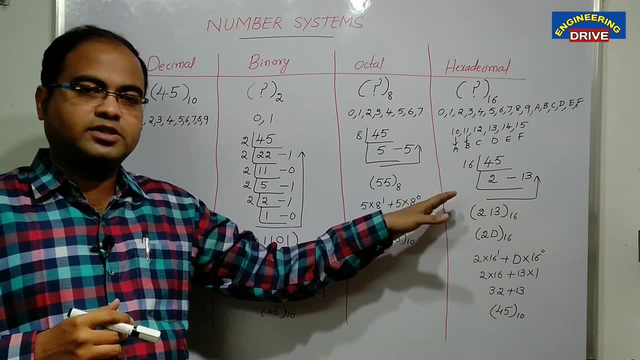 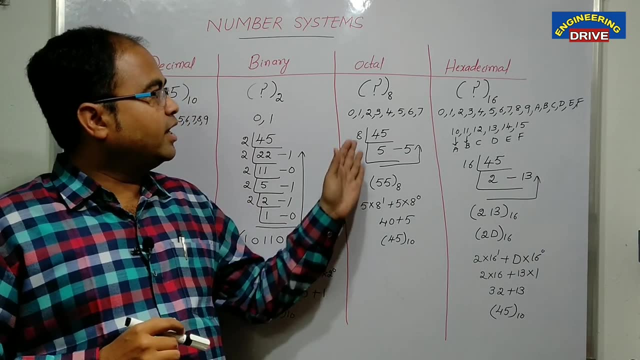 method where you can convert decimal to three different types of number systems, as well as from three different types of number systems to decimal. and the last question you can ask me is: sir, can, if octal number is given, can we convert into hexadecimal? yes, so what you should do first. 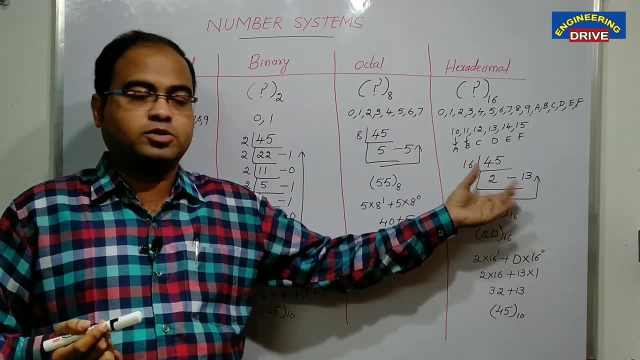 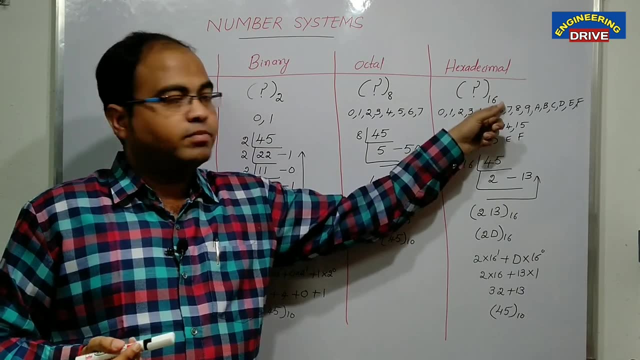 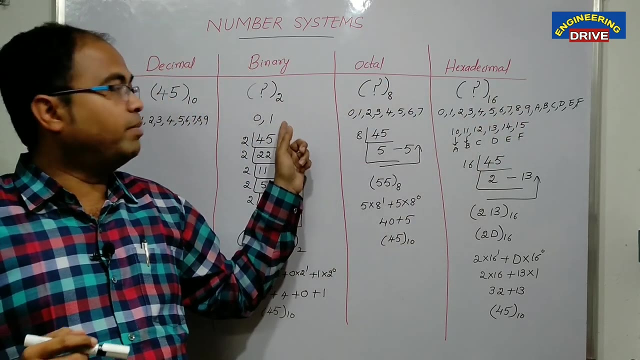 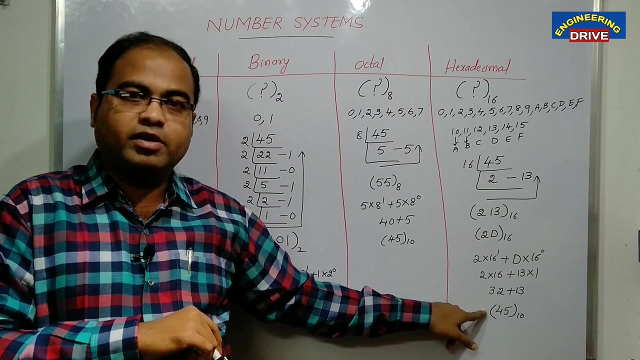 of all, don't convert octal directly to hexadecimal. it is not possible. first take the octal number, convert it into decimal number and then convert this decimal number to hexadecimal. okay, suppose you have. they have given in question. convert hexadecimal to binomial what you can do: first convert the hexadecimal number- let us say this 2d 16- into decimal number. 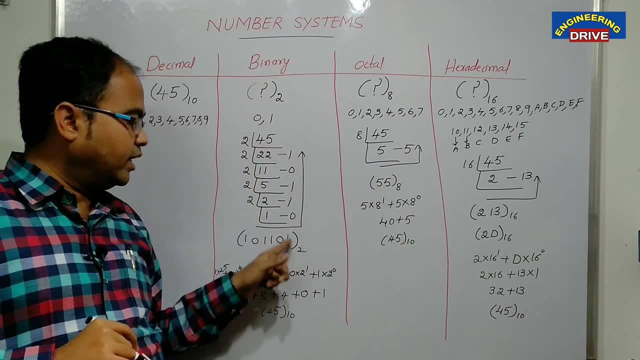 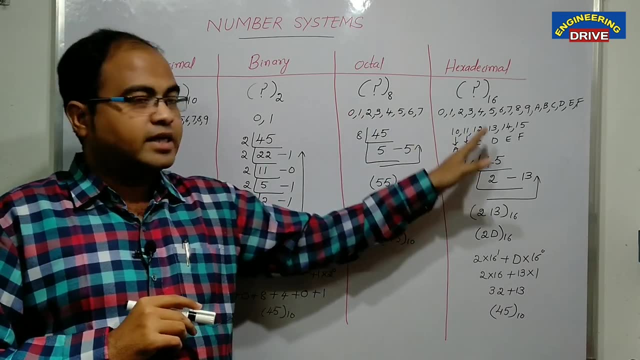 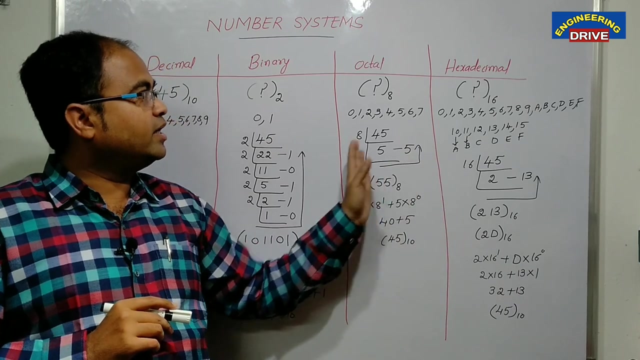 first, then convert this decimal number to binary like this. so direct conversion is not possible. it is very complex. so what you should do if any hexadecimal number is given: first convert the hexadecimal number into decimal and then you can convert either into octal or binary. so this are